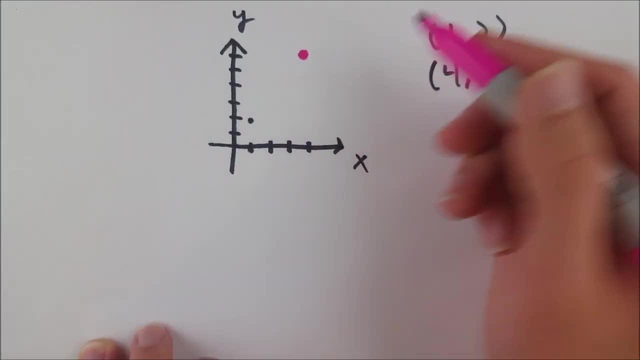 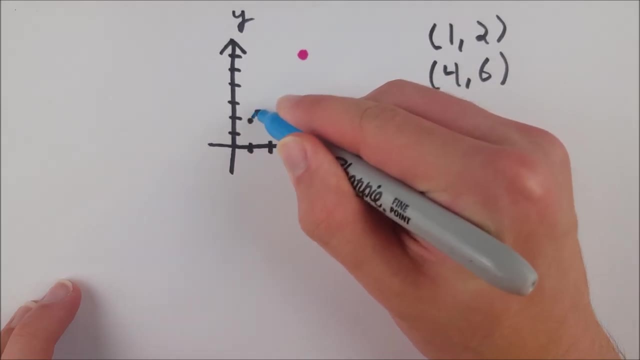 So these are our two points, That's 1, 2, and that one's 4, 6.. Could have color-coded it a little better, but oh well. So we are trying to find this distance between these two points. 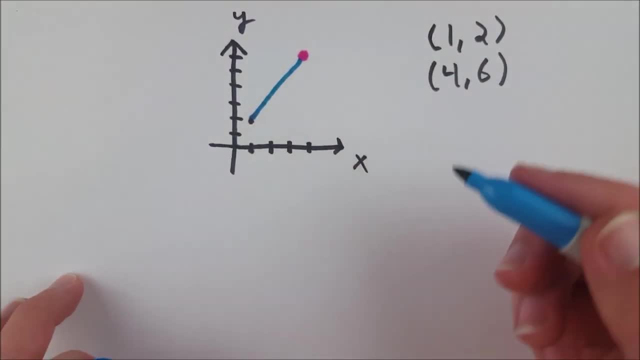 I'll just draw the segment. We're trying to find the length of that segment right there using the Pythagorean Theorem. So how do we do that? Well, to use the Pythagorean Theorem, of course we need a right triangle. 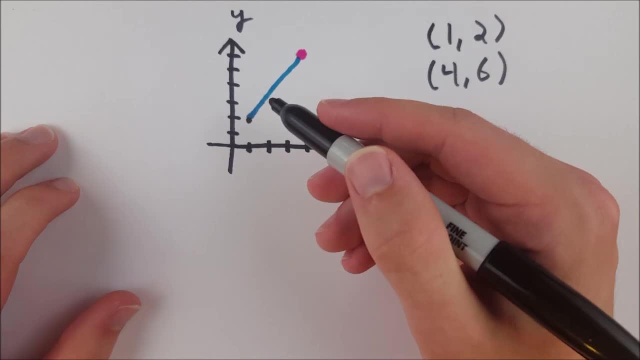 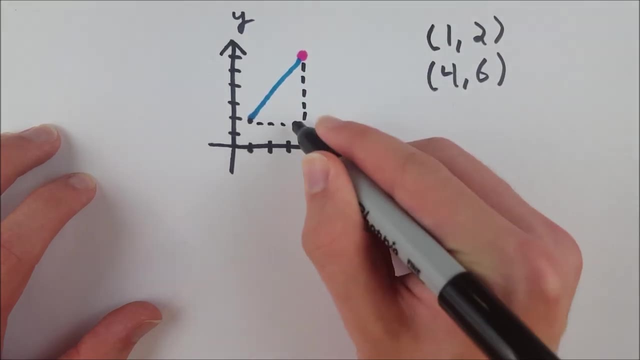 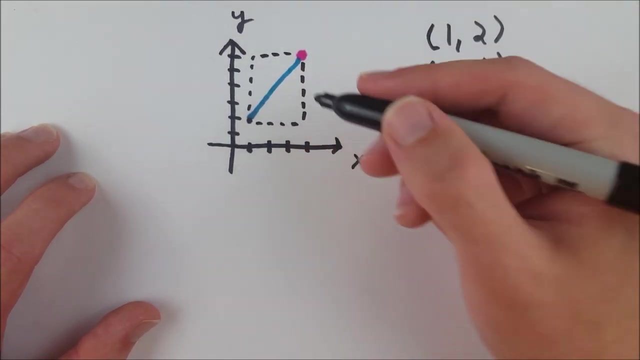 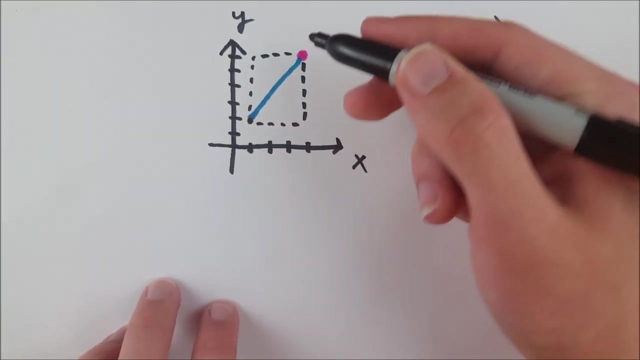 So what we can do is consider this segment as being the diagonal of a rectangle. The rectangle would look something like this, With the two points that we're trying to find the distance between as the two opposite vertices of the rectangle. So here's my decently drawn rectangle with our segment we're trying to find the distance of as the diagonal. 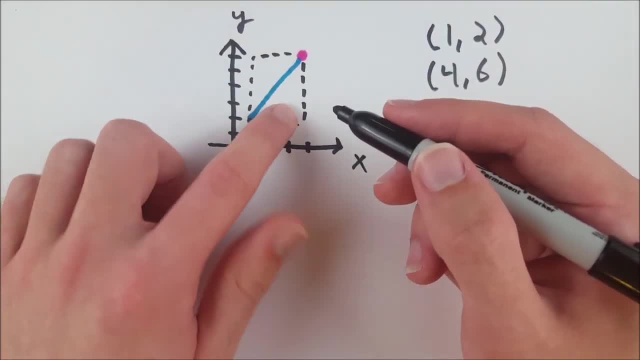 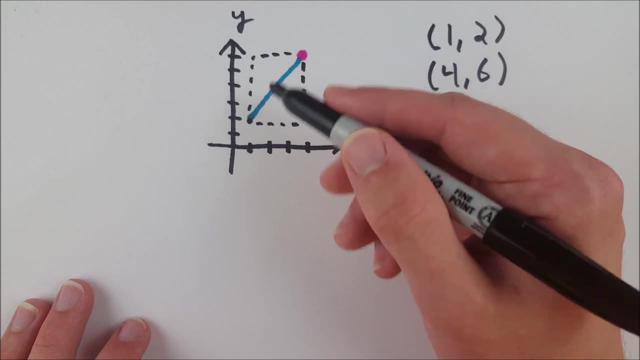 Now you can see we've got two right triangles, This one up here, this one down here. They're congruent. So from this point you can pick either right triangle you want, And we're of course going to use the Pythagorean Theorem to find the length of their hypotenuse. 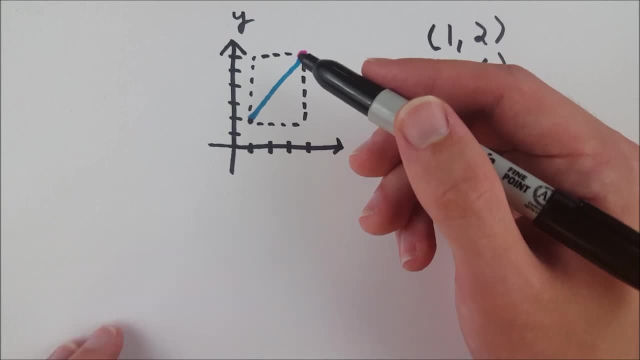 So pick whichever one you prefer to work with when you're doing a problem like this by yourself. For this example, we're going to choose this lower triangle, So we'll fill that in with a solid line. This is the one we're looking at. 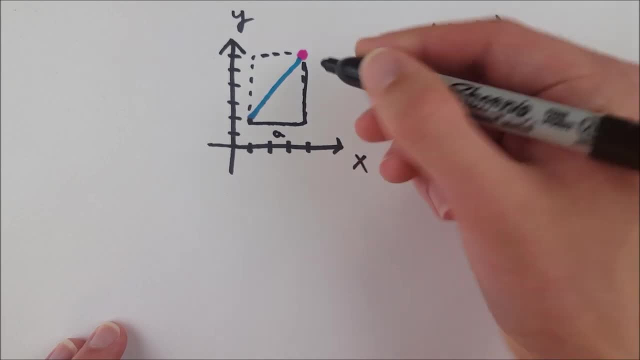 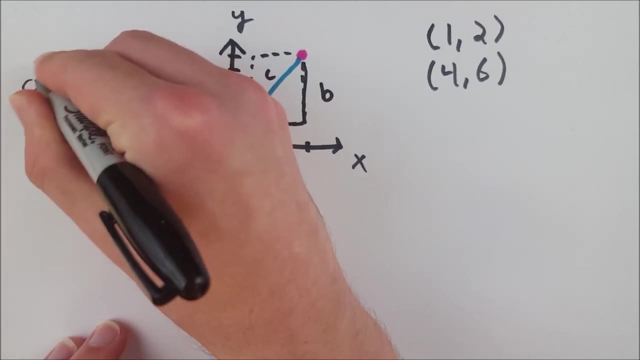 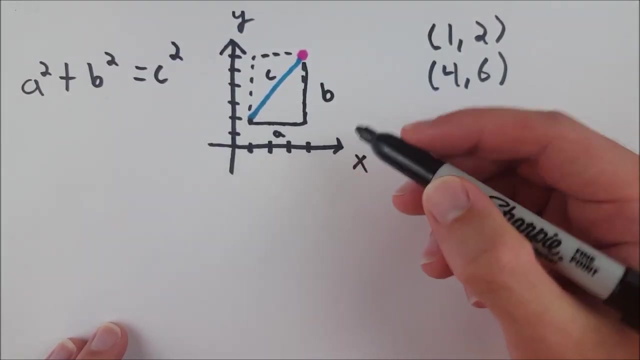 Now this distance here on this leg, we'll call it A, We'll call this distance here B And we'll call this distance here C. Remember that our Pythagorean Theorem is: A squared plus B squared equals C squared, Where A and B are the two shorter legs of a right triangle. 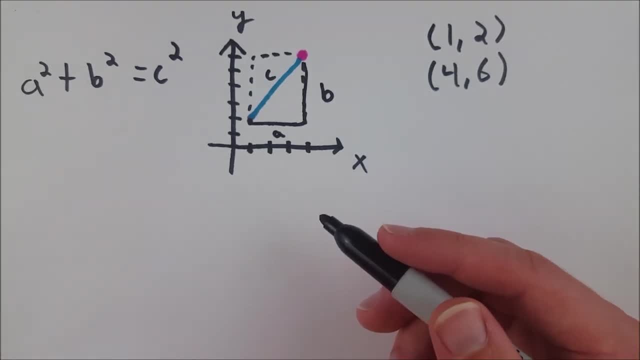 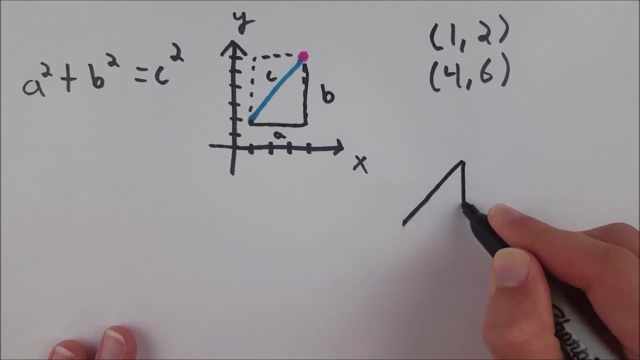 And C is the hypotenuse. The length of them, of course, is what we're talking about. So what I'm going to do now is just draw this right triangle outside of the graph, Because I like to work outside of the graph, where things are a little less messy, because there's not so much going on. 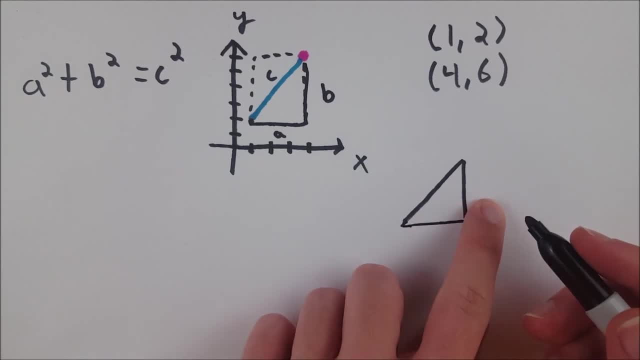 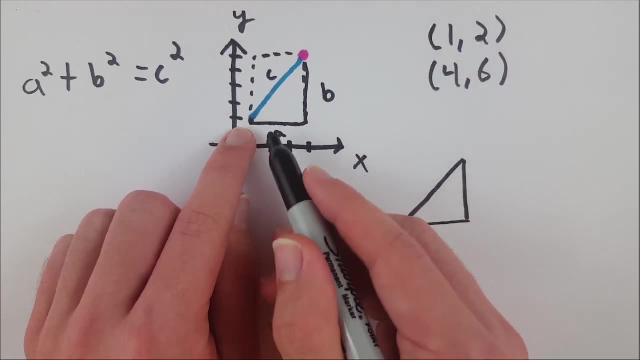 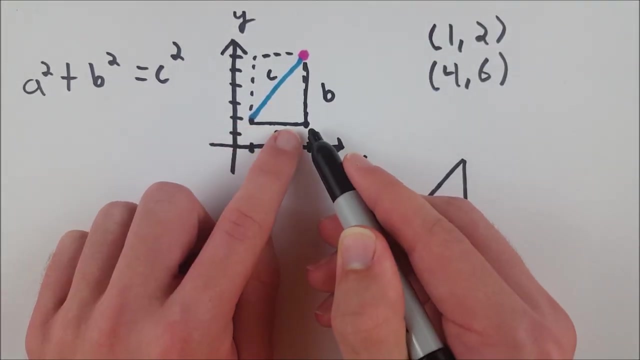 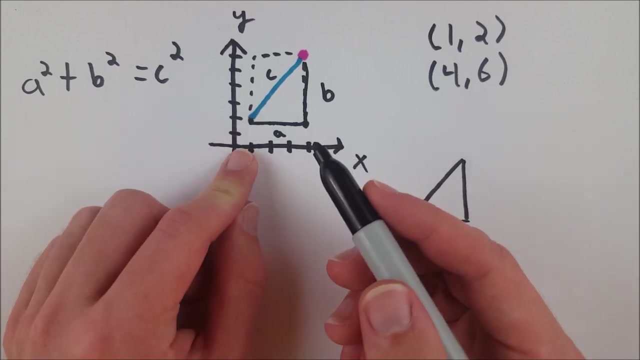 So here's our triangle And we're going to find the length of these legs. So this point right here, we know is Now we need to find the distance from this point to this point, because that would be the length of this leg. And we know that this point has the same y-coordinate as this point because we see they lie on a horizontal line just by construction, how we constructed the shape. 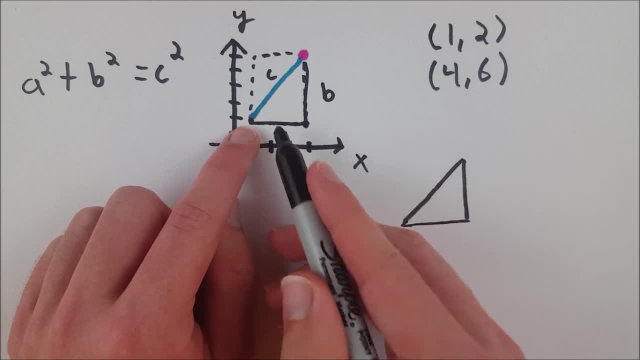 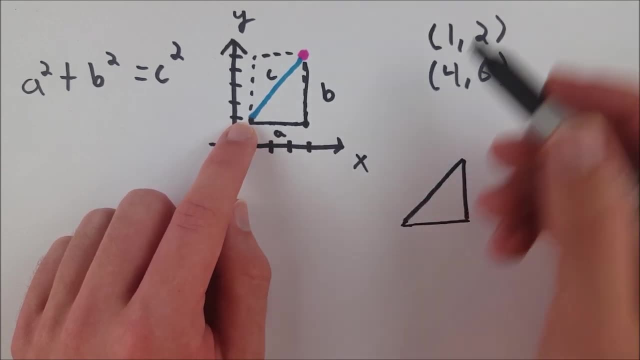 So, because they have the same y-coordinate, this one has a y-coordinate of 2 and this one has a y-coordinate of 2.. All we have to do to find the distance of this segment is: take the difference in the x-coordinates. 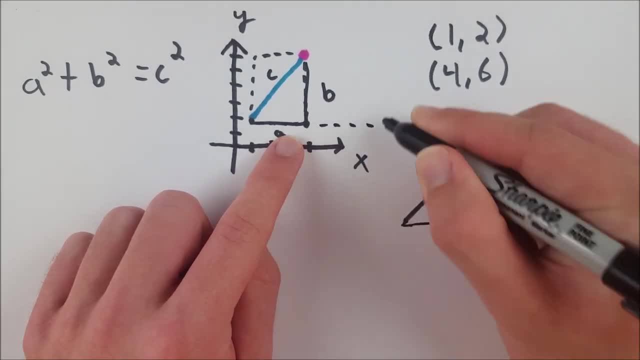 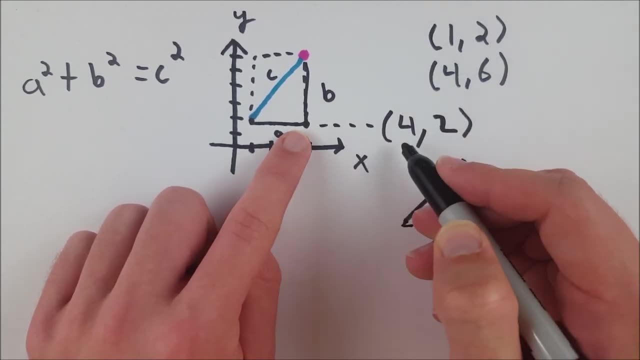 So this point is- let me write it out over here- has an x-coordinate of 4 and a y-coordinate of 2. So it has the same x-coordinate as this point up here and the same y-coordinate as this point down here. 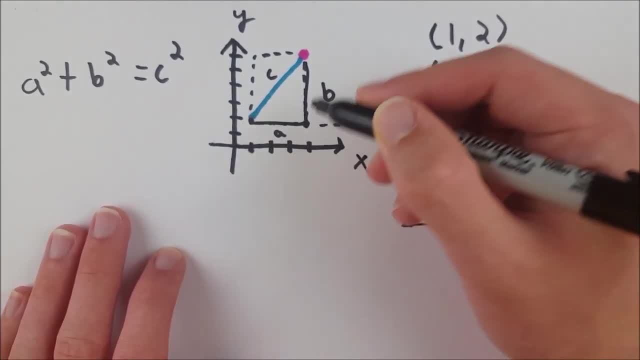 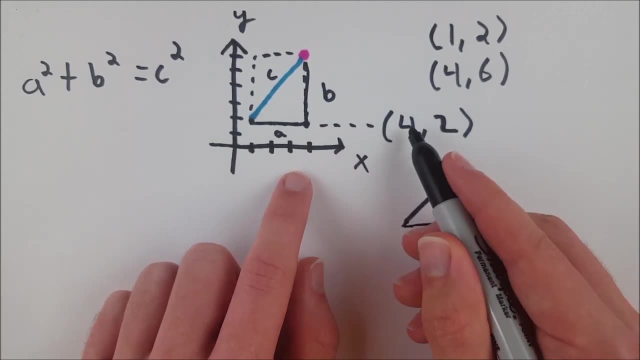 If we were on a full graph paper, of course you could just count lines, count the units between the points. You just count 1,, 2,, 3. And, as we see, that is the difference between the x-coordinates, between this point and this point. 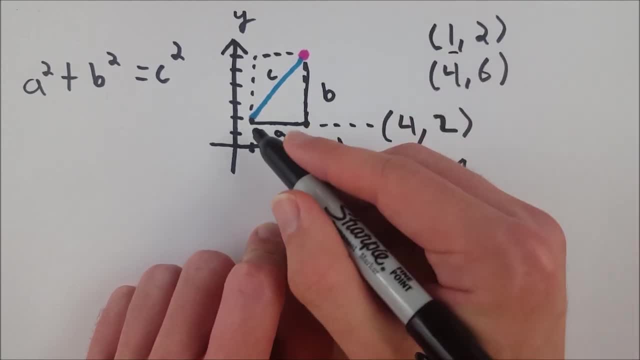 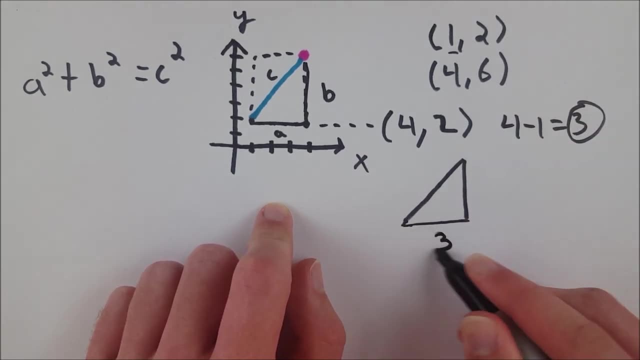 4, the x-coordinate of this point minus 1, the x-coordinate of that point, That's 4 minus 1, equals 3.. So 3 is the distance and that is the length of this segment. Same thing goes for trying to find the length of this segment. 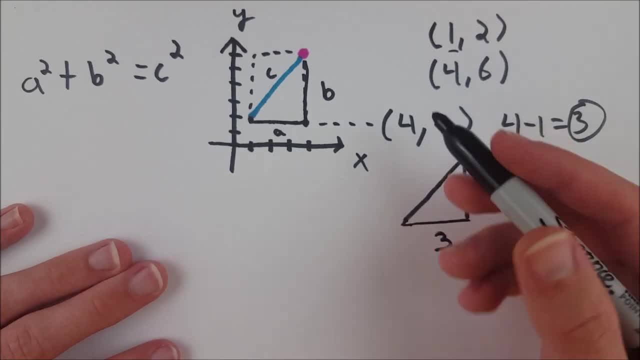 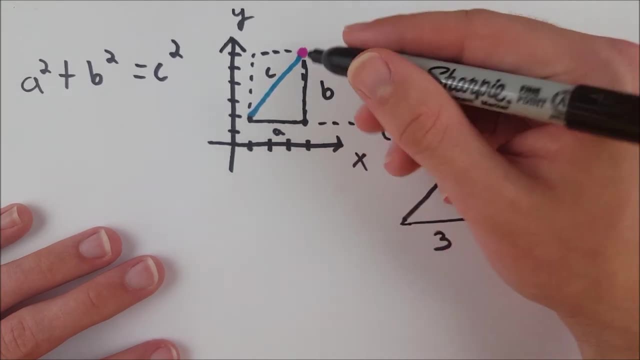 They have the same x-coordinate, each with an x-coordinate of 4. So all we have to do to find the distance is take the difference in y-values And again, we could just count up the boxes if we were on graph paper. 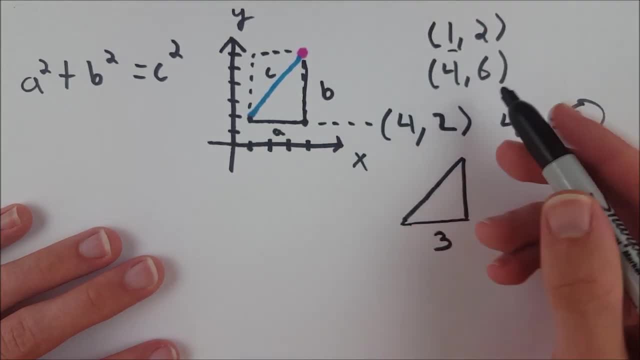 1, 2,, 3, 4.. And if we take the difference of their y-coordinates, that's 6, the y-coordinate of this point minus 2, the y-coordinate of that point, 6 minus 2, equals 4, just like we counted. 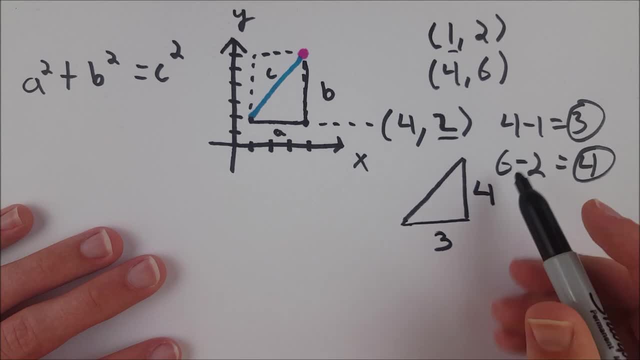 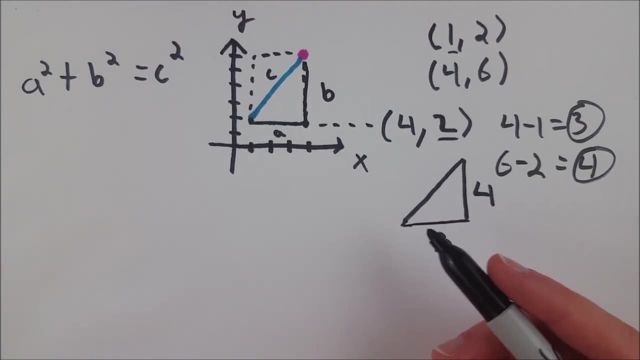 So the length of this side here is 4.. Now you could subtract these numbers in whichever order you pleased, But when you have a negative, you'll just want to make it positive. Negatives don't make sense when we're working with distances. 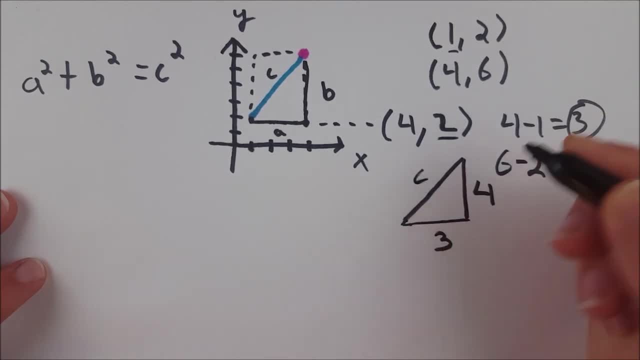 We're only interested in positive values. Now we're almost there. We're just trying to find c, now the length of this segment which corresponds to this c right here. So we just have to plug into our Pythagorean theorem here. 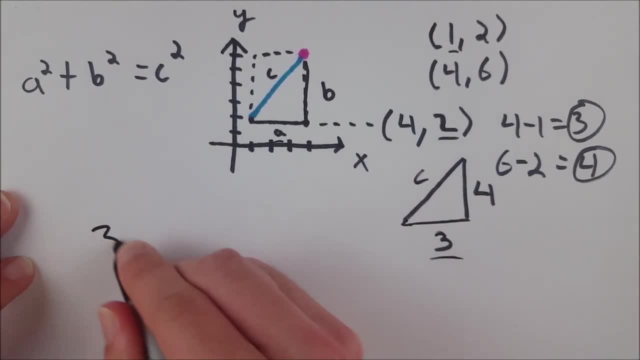 We know that this 3 right here is a, so that's 3 squared plus 4. right here is our b, That goes in b squared, so that's 4 squared equals c squared. Of course, this is one of the classic Pythagorean triples where we're working with all integers, which makes it very nice.